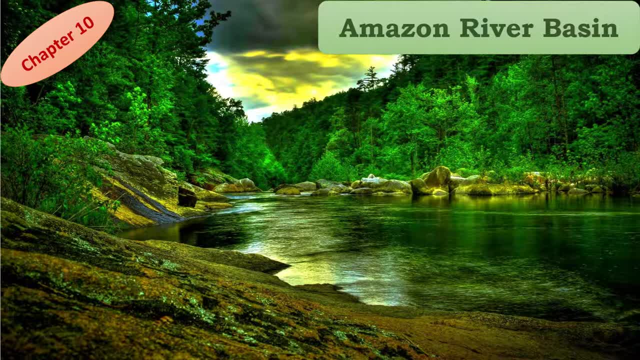 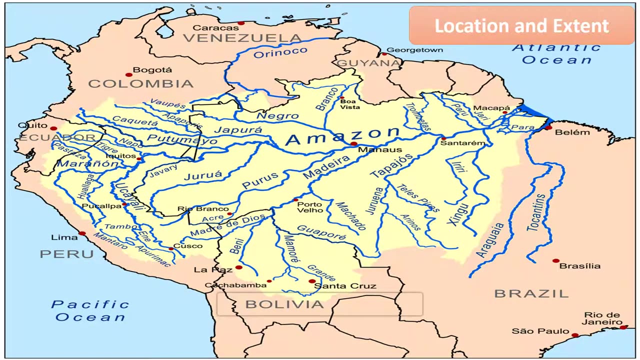 as the lungs of the earth. this basin is a part of South America. it is drained by the world's largest river, the Amazon, and its tributaries. now we'll discuss about the location and extent of Amazon Basin, as you can see on the map which is given. 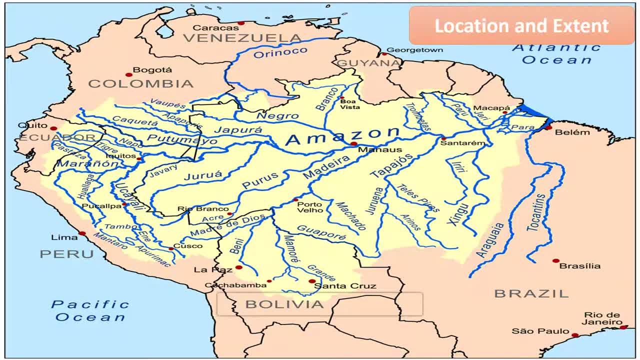 on the screen. the basin covers an area of about 75 lakhs kilometer per square. it covers about 40% of the total land area of the continent of South America. the Amazon River Basin is located in the countries of Venice and Manila, Suriname, Guana, Peru, Colombia, Ecuador, Brazil and Bolivia, the maximum. 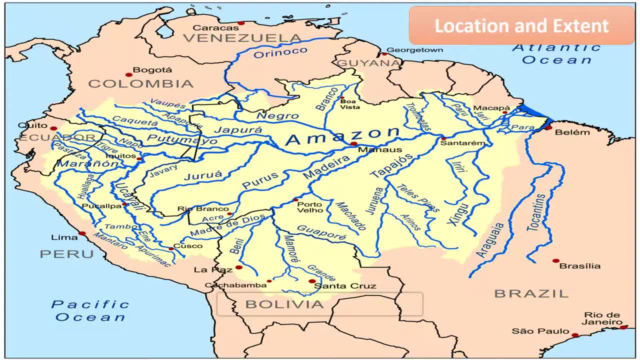 part of this basin is covered by the Amazon River rainforest. these rainforests are also called Amazonia. they are the largest and densest tropical rainforest of South America. on the earth. there are certain interesting facts about Amazon River Basin. let's have a have a look. the 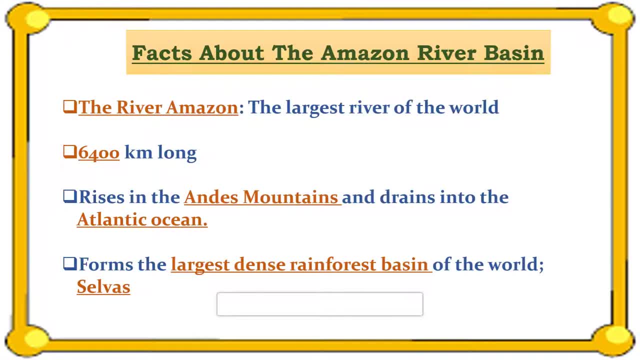 Amazon River is the largest river of the world. it is about 6400 kilometer long. the Amazon River rises in the Andes mountains and drains into Atlantic Ocean. it forms the largest dense rainforest basin of the world. and the last point, that is, the dense rainforest basin of South America, is also called Selvas. now we'll discuss. 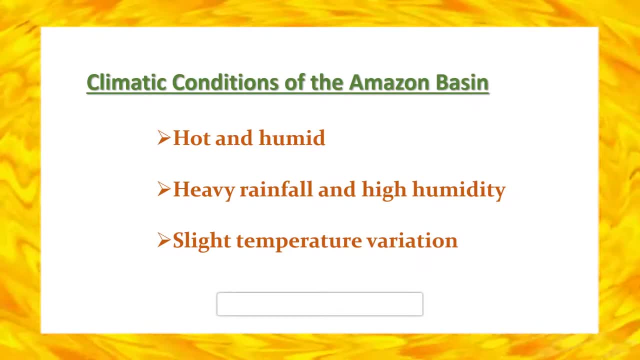 about the climatic conditions of Amazon Basin. so there are three important points, students, which you need to remember. first one, that is, the climate of Amazon Basin remains hot and humid throughout the year. second one, that is, it is characterized by heavy rainfall and high humidity. and the third one, that is there is a slight temperature variation in the 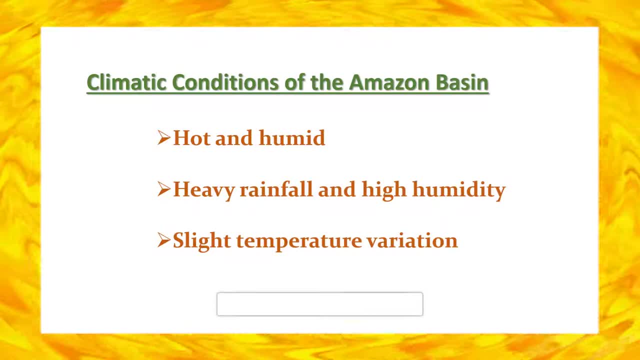 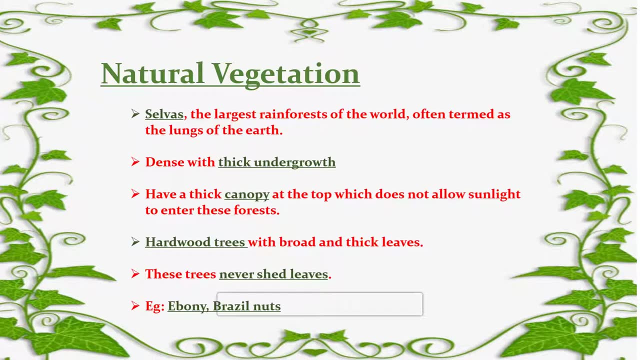 area as it is located near the equator. now we'll be discussing about natural vegetation, so the dense equatorial rainforest basin is also called Selvas, as we have already discussed in the previous slide. they are the largest rainforest of the world. they are often 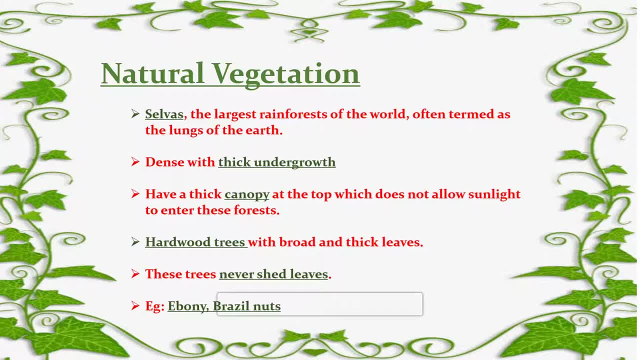 termed as the lungs of the earth. these forests are very dense with thick undergrowth. they have a thick canopy at the top which doesn't allow sunlight to enter these forests. these forests have hardwood trees with broad and thick leaves. these trees never shed their leaves at a particular season. 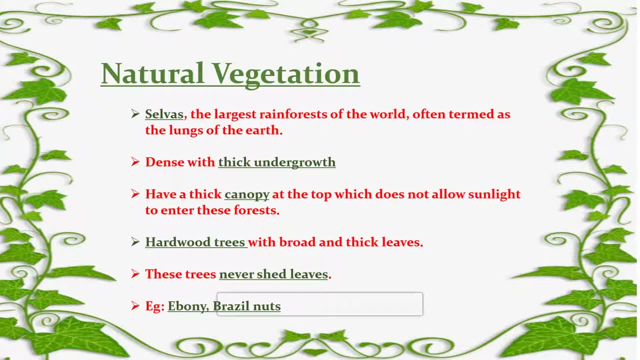 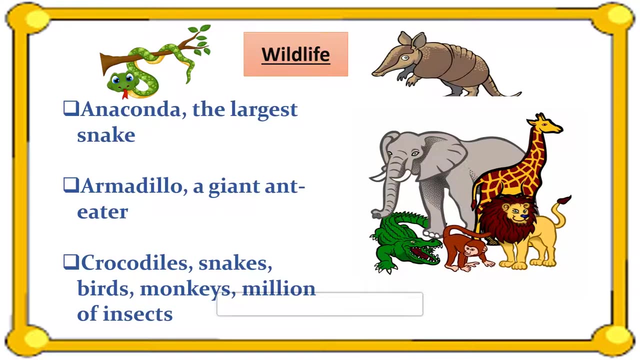 Therefore, these forests are called evergreen forests. Now, the examples of some important trees of equatorial rainforests are Brazil nuts, ebony, etc. Now let's have a look on the wildlife of Amazon basin. So the Amazon basin provides shelter to variety of wild animals. 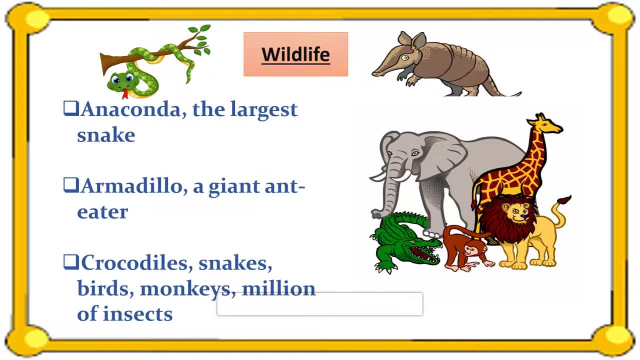 So we are going to mention some of them. It is home of anaconda, the world's largest snake. The armadillo, a giant ant eater, is also found in the equatorial rainforests. Now, apart from these animals, crocodiles, snakes, birds, monkeys and millions of insects are also found in these forests. 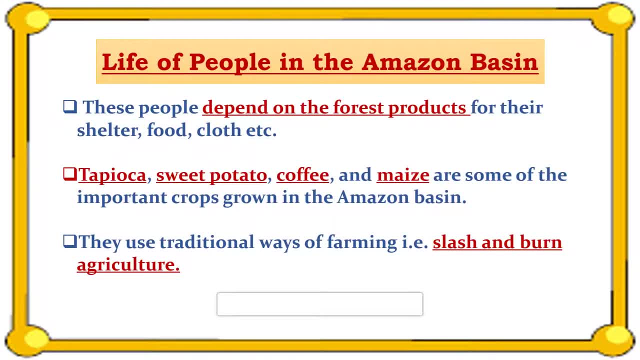 Now we are going to read about something about the life of people who live in the Amazon basin. So the Amazon basin is a home to about two million people. Most of them follow traditional way of living. These people depend on these forests for their day-to-day life. 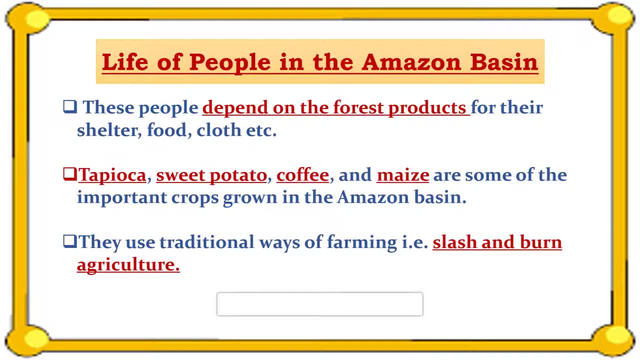 These people depend on the forest products for their clothes, shelter, food, etc. They use traditional ways of farming. They are indulged in slash and burn agriculture, which is very harmful for the environment as well. Now, tapioca, sweet potato, coffee, cocoa and maize are some of the important crops grown in the Amazon basin. 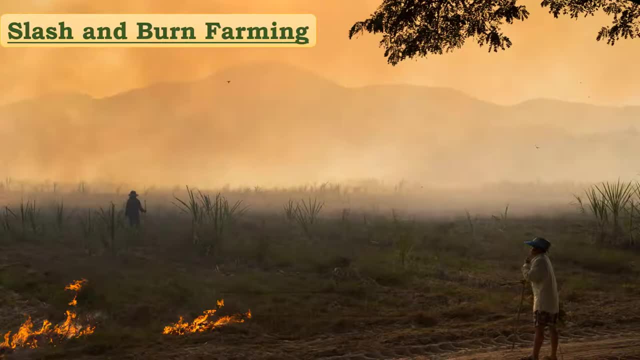 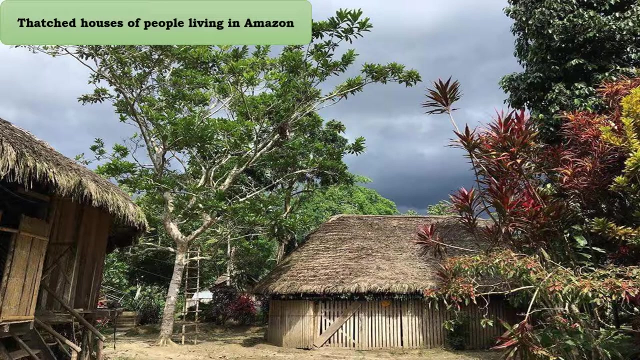 Now these indigenous people, as you can see on the screen, slash and burn. farming, which is a traditional way of farming, is also used by the people who live here And, apart from that, they live in thatched houses. People live in the thatched houses in the Amazon basin. 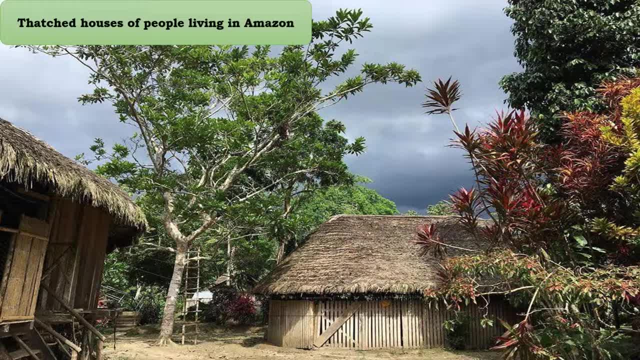 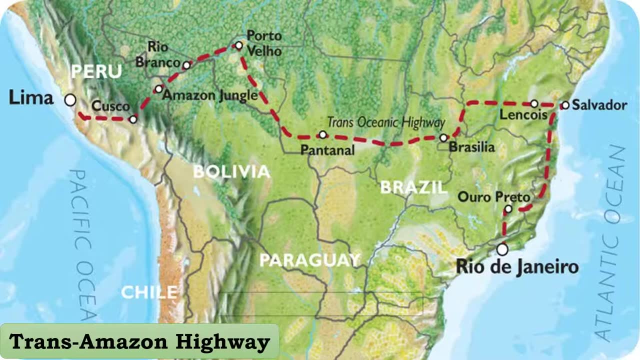 These indigenous people. they make this kind of houses. Now, in 1970, what happens? the Trans-Amazon Highway was introduced for an easier access to the Amazon. In spite of the presence of all the above, you know, discussed features, you can see on the screen Trans-Amazon Highway, which is shown on the map right.